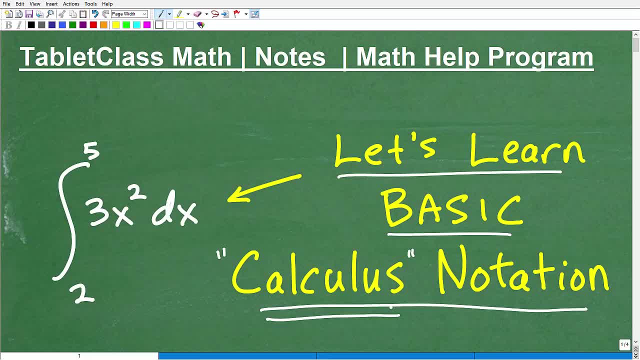 people, if anything else you know for this particular video, you really truly have to appreciate the impact mathematics uh has in your modern day life, and probably nothing as is as impactful as calculus. so we're going to talk about this basic notation here in just one second, but first let me quickly introduce myself. my name is john. i'm the founder of taba, class math. i'm also 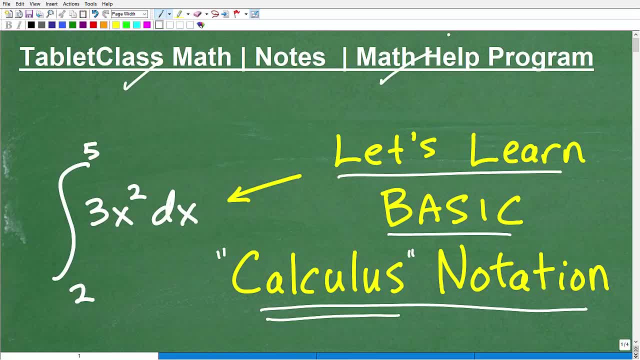 a middle and high school math teacher and over several years i've constructed, but i constructed what i like to believe is one of the best online math help programs there is. of course, i'll let you be the judge of that uh statement. if you're interested, you can check out my math help. 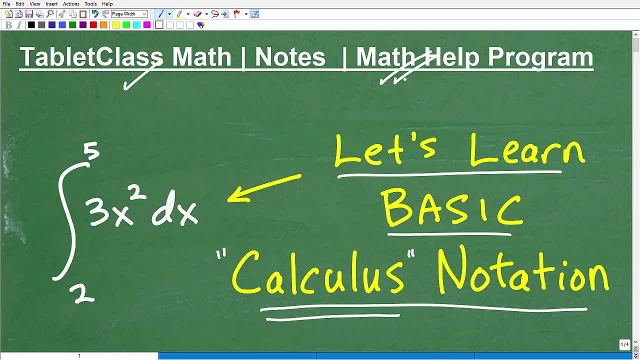 program by following the link in the description of this video. but basically i offer 100 plus different math courses. i have all the main courses, uh, for middle and high school math, like pre-algebra, algebra 1, geometry, algebra 2.. i'm going to be launching. 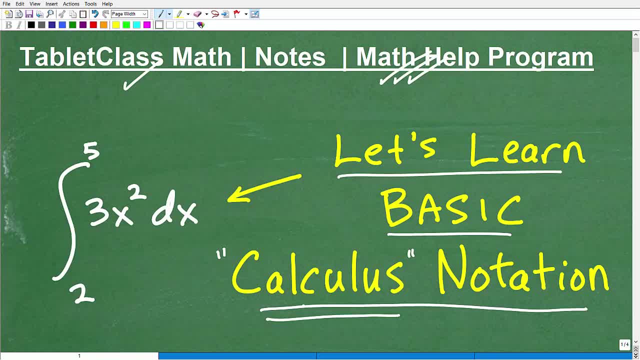 pre-calculus here shortly and that is obviously the course you need to take before you take calculus. so if you're interested in that, check back about a month from when i'm posting this video and my course should be launched. but i also do a lot in the area of test preparation, i think. 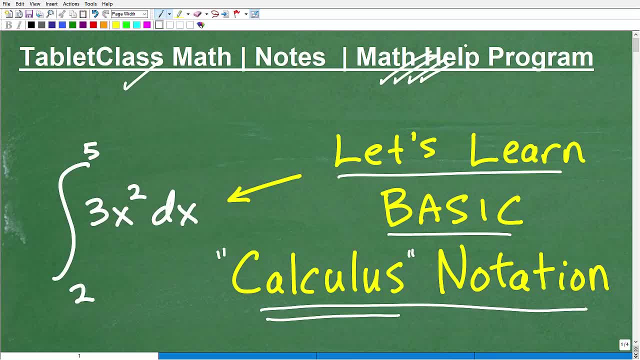 i'm going to be launching a lot of things like: uh, for those of you who are studying for the ged, sat act, gre, gmat, asvap, alex accuplacer, uh, clep exam, teacher certification, nursing entrance- there's a million different reasons why people study mathematics outside of a formal math course, so 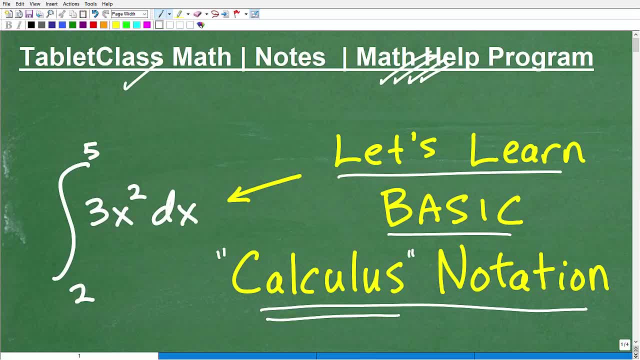 if you're studying for any particular exam like that, go to my site again. you can find the link in the description of this video and check out my course catalog. i should have that if i don't drop me a line in my contact form to help you out the best i can. 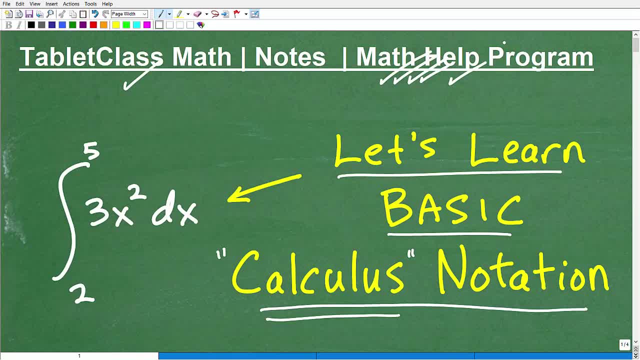 i also work a lot with independent learners like homeschoolers, so if that's your situation, i have a great homeschool learning program and then obviously help those of you who are just having a difficult time in your math class. but one thing you need to do if you are studying mathematics: 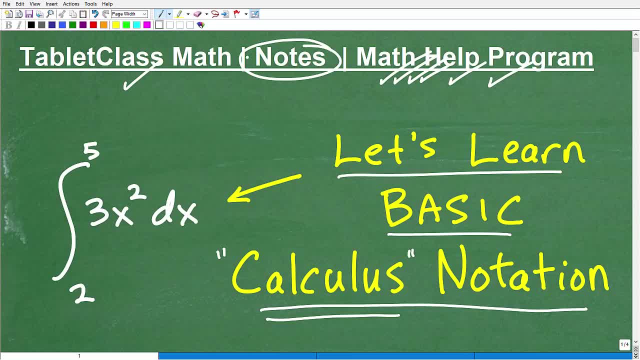 that is, take great math notes. so, over decades of teaching mathematics, one thing is apparent to me: those students who take great math notes will be successful in mathematics, and those of you that don't take math notes are like: yeah, i don't want to do that, just like me. 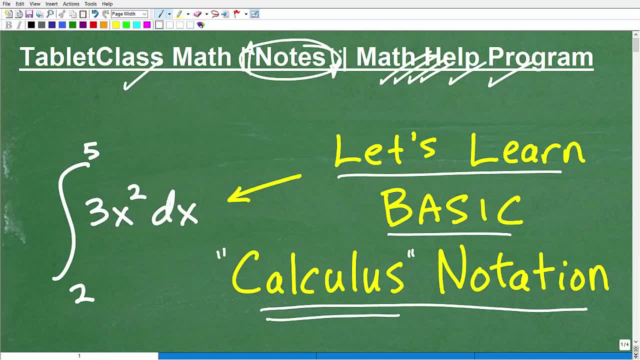 back in the 1980s and i'm like, yeah, i won't do that and guess what my grades suffered, until i figured out that you know what note taking that is an absolute requirement. the better your notes are, the better your grades are going to be. but if you are in a particular math class and you don't have 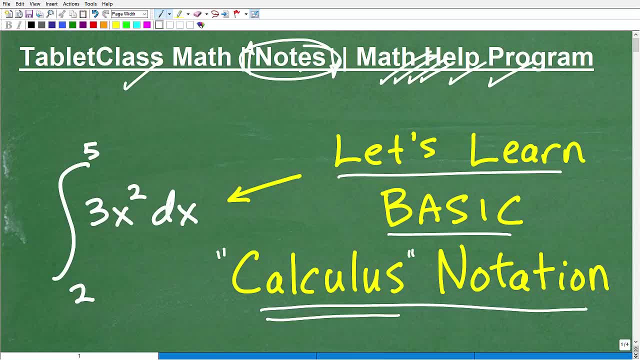 good math notes. right now you need to start working on that, but i offer a detailed, comprehensive math notes you have something to study from to include pre-algebra, algebra 1, geometry, algebra 2 and trigonometry. find links to those notes in the description of this video and i'll see you in the next video. 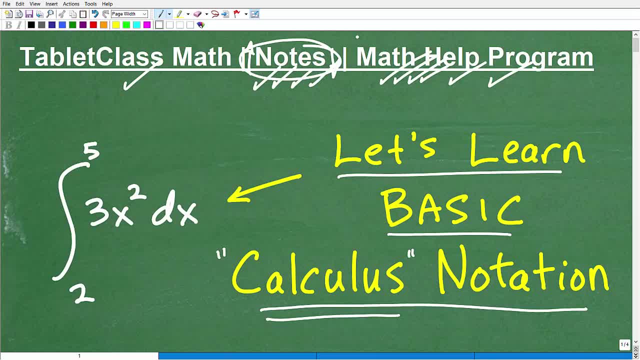 all right, so let's get into calculus. and you know it's funny because i uh when you're there's different movies that i've watched through the years and they'll have some math. uh, you know, there might be some mathematics going on, whether it's a code breaker or some sort of 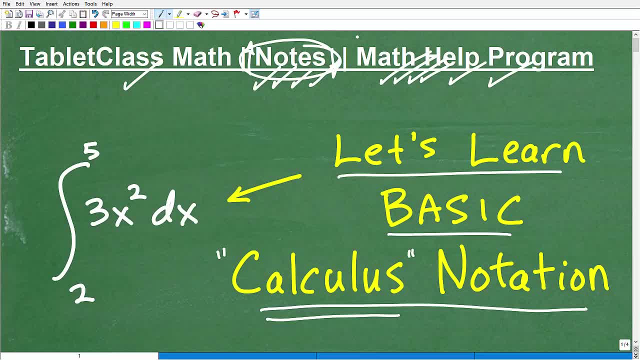 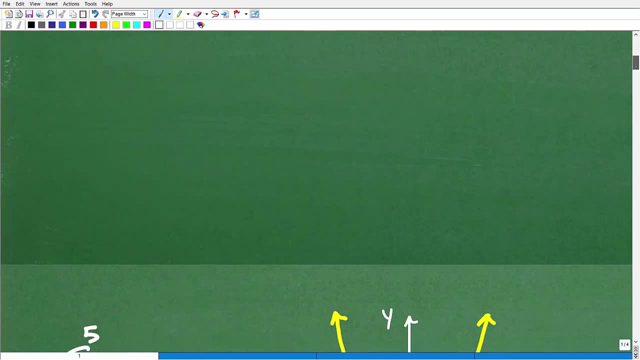 you know seeing, and you'll see some calculus and of course, as a math guy, i'm like: oh wow, look at that. you know it looks so advanced and just, uh, you know crazy stuff. but this is what calculus looks like. this is a pretty basic kind of calculus problem and let's discuss this notation, okay. 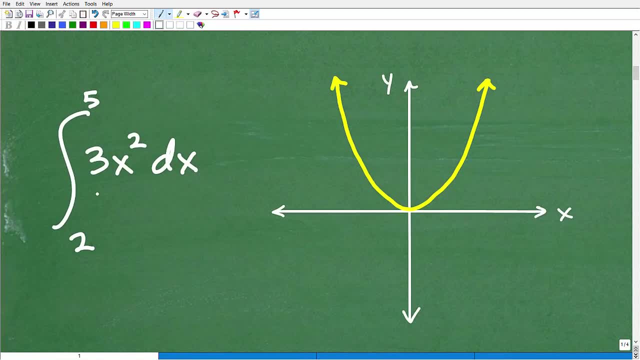 all right, now this calculus, what i'm talking about? this would be something that you would take as kind of an introductory calculus course. all right, so i have a graph going on here and now let's just talk about these symbols. so the first symbol that might come to mind is this whole little long thing. 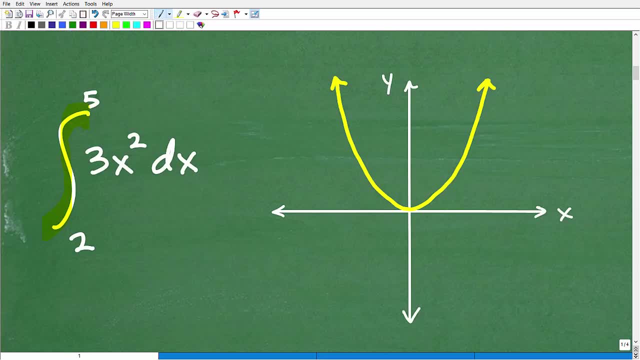 right here. this is a kind of very common calculus symbol. this guy right here and that's referred to as an elongated s all right. so debt like s like this, the the letter s now. now, if you elongate, that s right, it's going to kind of look like that. so this is kind of what. 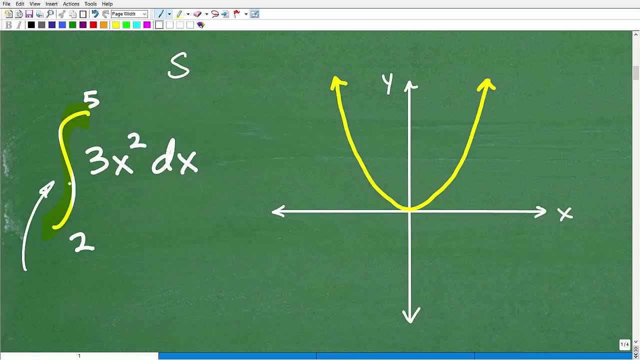 that is, and you can kind of think of this elongated s as part, or it's related to this word sum. okay, because that's basically what it means. all right, this means we want to find the sum. we want to do what? well, the sum is, what we get is the sum of the number, right? so e t i sometimes work on. this because, if you have, if you don't know what z is, it's essentially the sum of the temperature and you want to find the number in the room. so z, you want to find each zone and you measure the temperature um tonight 없이. you want to find the number because we have to find each zone and you level it all in. 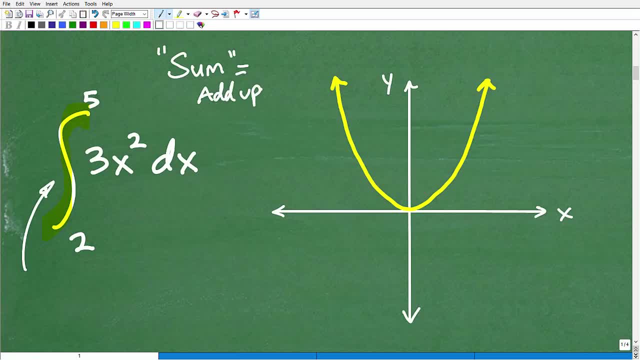 what add up? we want to add some things up, and that's what this symbol basically is: stating: hey, we want to add some things up, all right, we want to find the sum of what? well, that's our next thing right here. okay, now this 3x squared this. 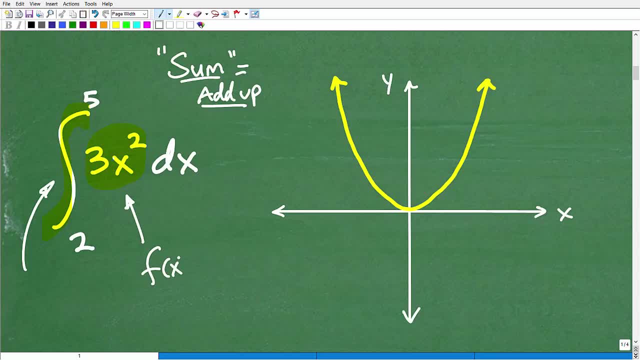 is an example of what we call a function in mathematics and this is kind of the kind of general symbolic symbology or notation for a function and what is a function? right? so this is a specific function: 3x squared. but if I wanted just to write a generic function, I just say I have some function. I would just write: 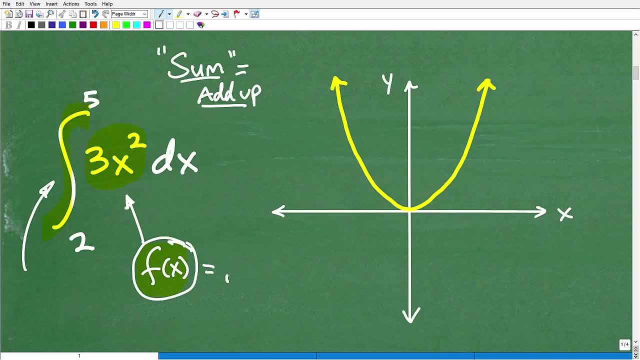 this symbol: okay, but what is a function? well, a function is effectively a rule, okay, and it has an associated graph with it. so this function 3x squared, okay. now, for example, you can see that the function 3x squared is a function that has an associated graph with it. so this function 3x squared, okay. now, for example, 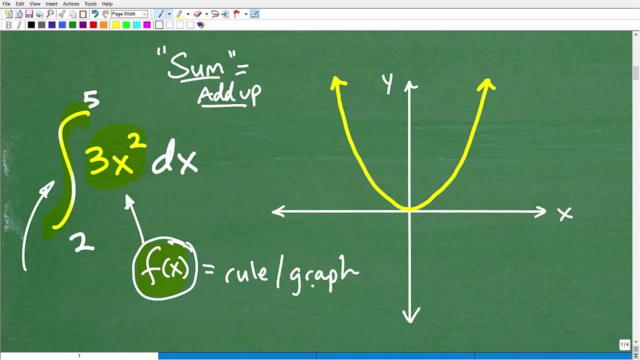 could be this graph right here. okay, this could be the graph of this particular function, so we'll just call this our function: 3x squared. and for those of you that might know some basic algebra, this is what we call a parabola. it's a. 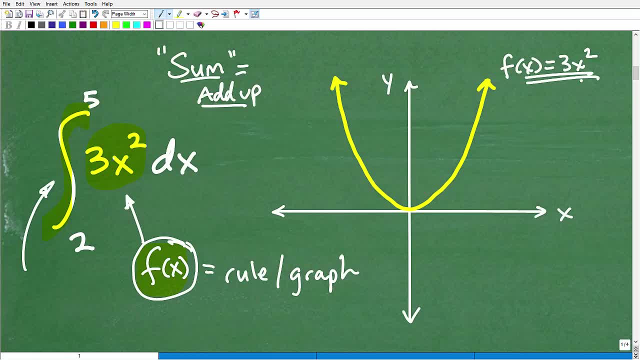 u-shaped graph, and this is how we kind of basically describe it. okay, now, all you need to know is that 3x squared graphically looks like this, and this is just some basic algebra. it's not that difficult to graph these things. so what do we have so far? well, we want to add up, okay, we? 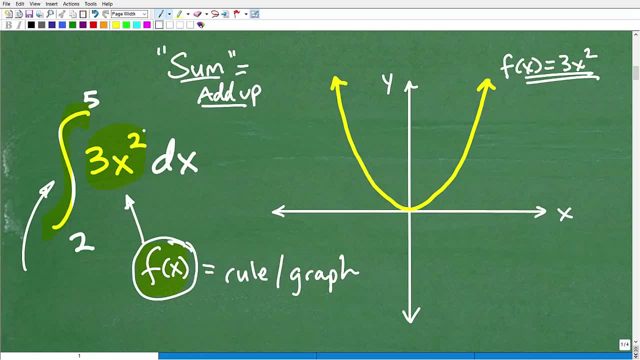 want to find the sum. we want to add up some stuff that is somehow related to this particular function or this particular graph, right? so that's what we're at so far in our nice little calculus exploration. so the next question is: well, what do we want to add up? okay, what are we trying to find? the 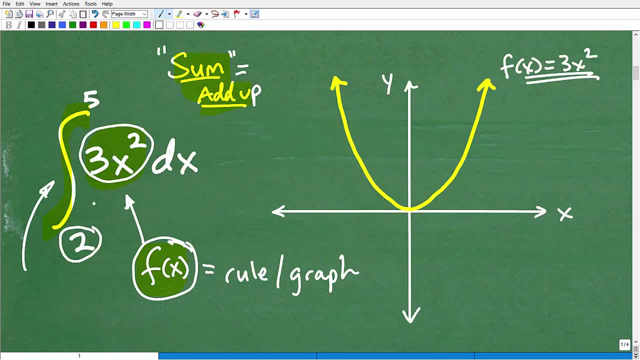 sum of. well, that's where these little numbers right here are going to come into play. so we have 2 and 5. well, these guys right here, 2 and 5, we're going to be associated with this x-axis. now, if you're not familiar with a, 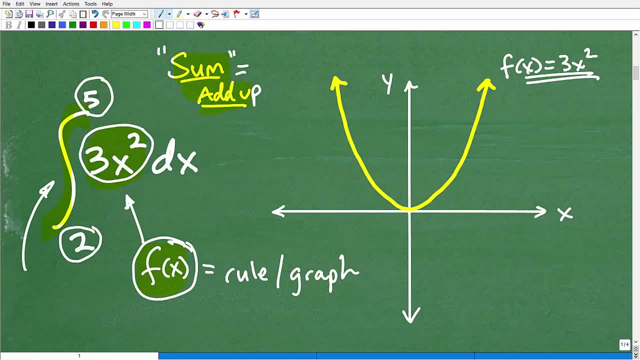 basic xy-axis. the way it works is this: this is 0 in the middle, and then this is 1, this is 2, this is 3, this is 4, this is 5, and you kind of get the idea. so this way it's the negative values: negative 1, negative 2. negative 3. negative 4, negative 5. 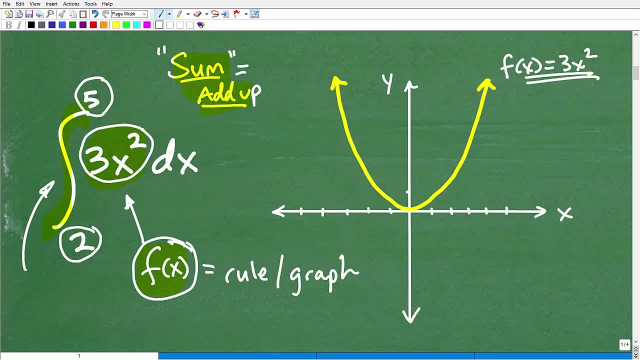 and then from right here on the y-axis, this is a positive 1, 2, 3, 4, 5, just goes on and on and on: negative 1, negative 2, negative 3, negative 4, negative, 5. so this is a basic xy plane and we use this standard plane here, this xy graph, to 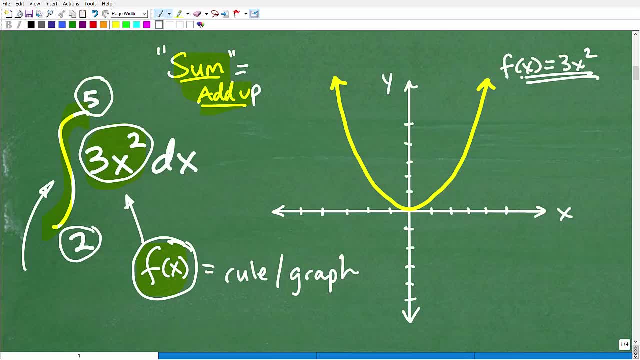 graph our functions. okay, all right. so let's get back to these guys right here. this 2 and 5, these are boundaries on the x-axis. so let's go to 2, okay, and let's go to 5. so that's 1, 2, 3, 4, 5, okay, so what we're? let me move this over here because I'm gonna 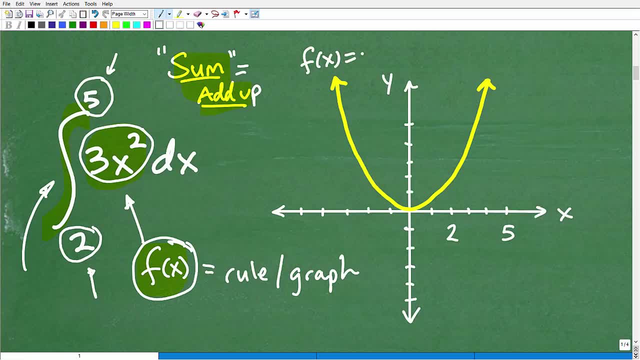 have to draw or sketch here. so here's our function again. all right, so what we're trying to do is, in calculus, what is a very common goal. okay, in calculus, basic calculus, we call integration. so integration just effectively kind of means to add up. now of course I'm kind of simplifying, or 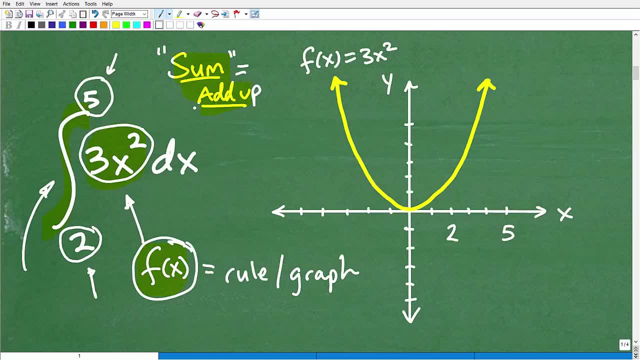 oversimplifying, as some of you out there like. no, no, it means specifically this. that's that's at the point. I'm not trying to teach to to you in a very technical way, I'm just trying to give you some general feel for this. so integration is kind of add up. so what are we going to add up? well, we're going. 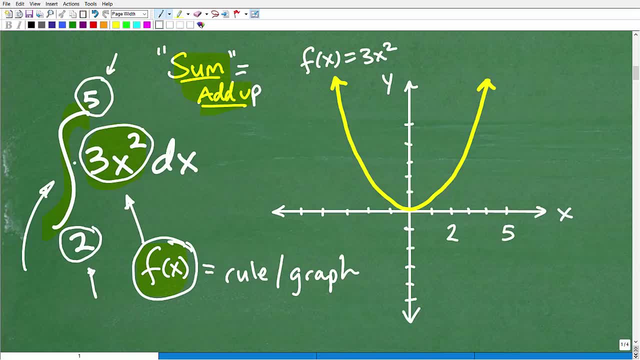 to add up this, this particular function. but what does that mean? well, for us, we want to find the area underneath this functions graph. so here let me show you what that looks like. so, from here, from 2 to 5, actually, let me draw this out a little bit more. okay, so that cuz, this graph continues on, and on, and on. 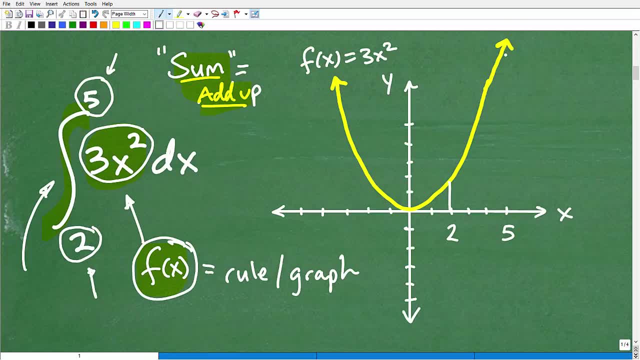 okay, alright, so from 2 to 5. alright, in calculus, what we wanted. oftentimes, when you're doing this type of of problem, what we're trying to do is find the area. okay, underneath the curve, underneath a particular function's graph, okay, and it's kind of bounded. from here it's going to go under the graph. 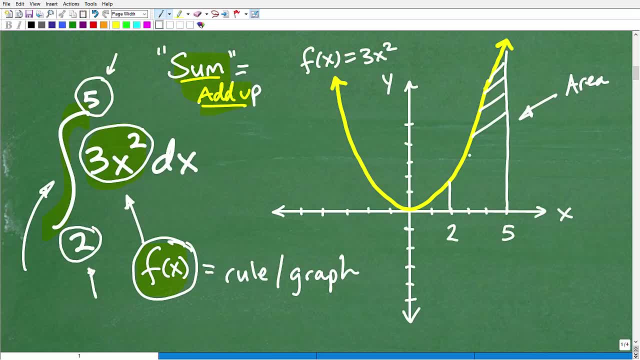 just like this. all right, so this is what we're talking about like. so, all right, so we're this particular um, uh, integration problem. that's what this is called. okay, we want to add up from two to five underneath the functions: graph 3x squared. that's what we're trying to do here, right? so this? 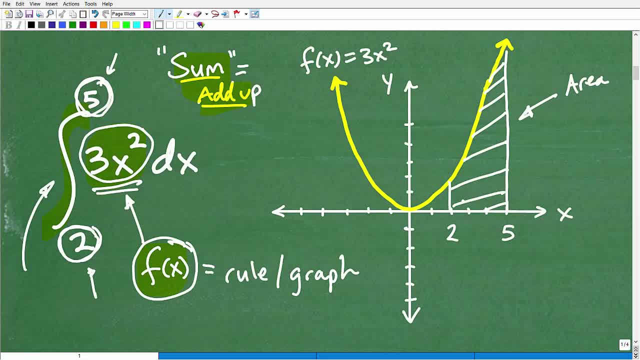 is kind of the main idea of this particular calculus problem. now this little dx is related to another topic, a very, very hugely important topic in calculus, called the derivative. but for now you just need to know that that's a a little notation that we write when we do this type of. 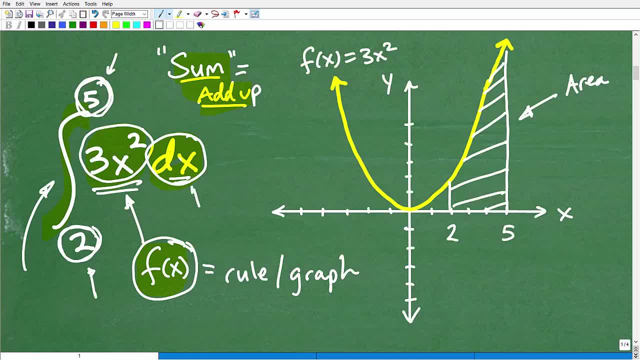 problem. okay. so that's all this means right here, all right, so we kind of not really focus in on it so much for the purposes of understanding this particular problem, okay. so, uh, what are we trying to do here? well, we're so far. what we want to do is we want to um find the sum okay, or integrate, we want to add up um underneath. 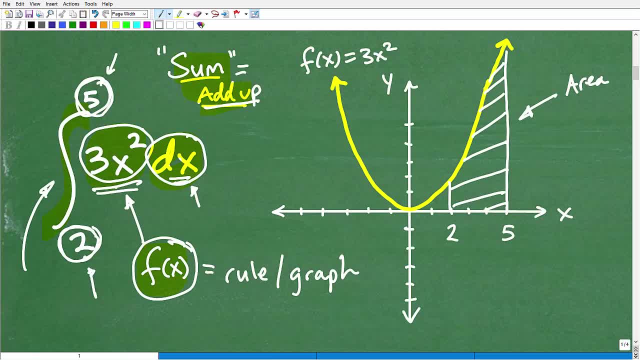 the curve between two and five of this function's graph. all right, that's basically it. if you're with, you're doing our homework. you're not really working automatically right now. you're not really thinking about adding up. we're talking about adding up up, all right. so you might be saying: 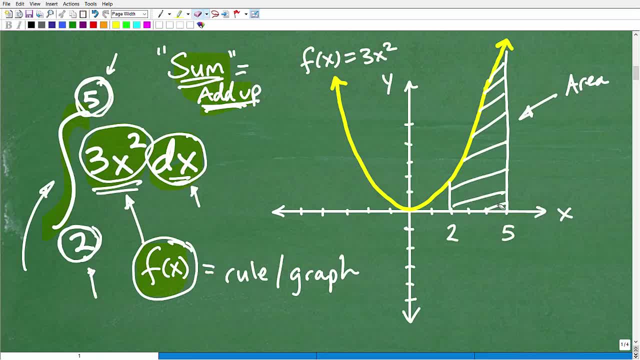 yourself. well, add up what. well, let me kind of explain to you what we're talking about, okay? so let's go back to this uh problem here. if i wanted to find the area underneath the this shape here, i could be like, hmm, you know what i'm gonna give. 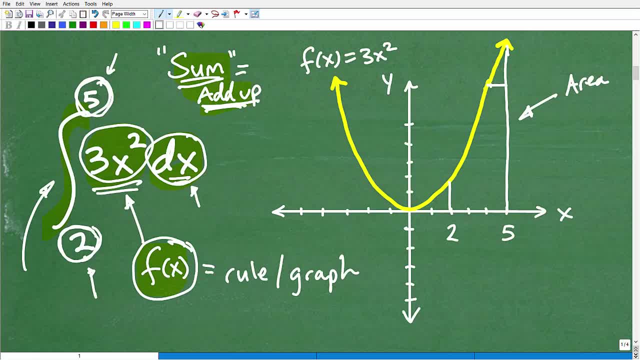 give. i'm going to give myself an estimation. i'm going to go like this: i'm going to make some rectangles, all right, because i don't know how to do calculus, i don't know the procedure here, right? so, um, i might just make myself some rough rectangles like this, and everyone knows how to. 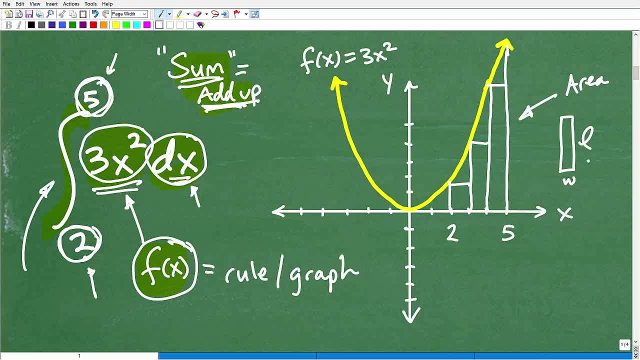 find the area of a little rectangle. it's just the length times the width, right? so if this was 10 and my width was 2, the area of this little little strip here would just be 20, 20 units, uh, squared. okay, so i could find, uh, this area, and then i can find this area and i can find this. 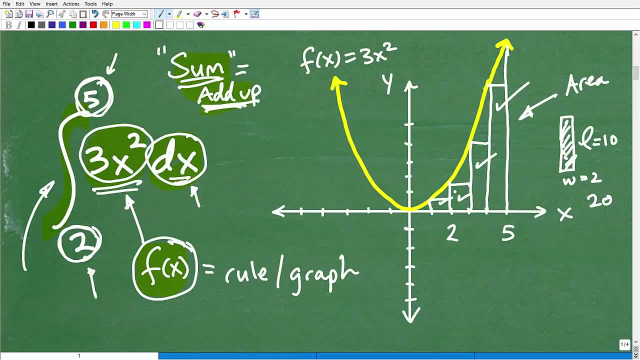 area and let's put a little small one right there. i could find that area right there, okay. so if i add up, right, if i find the sum of this guy, this guy, this guy and this guy, all right, i'm going to have some basic idea of the area underneath this curve, right. so this is kind of where this is going. 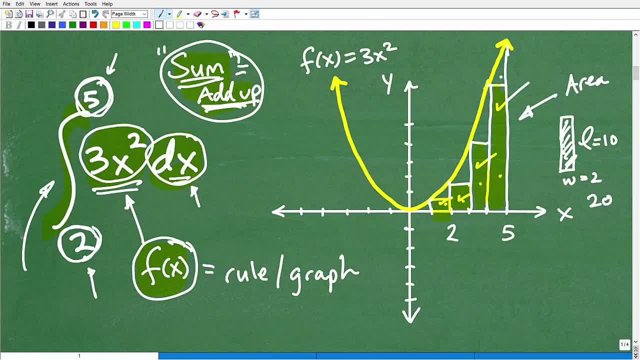 but that's just a basic uh, you know, we're still missing, like look at all the gaps we have here. so that's, you know, that's a pretty good idea, but how could we make our answer more precise? well, we could add up what? well, we could add up smaller little strips. okay, things that we can. 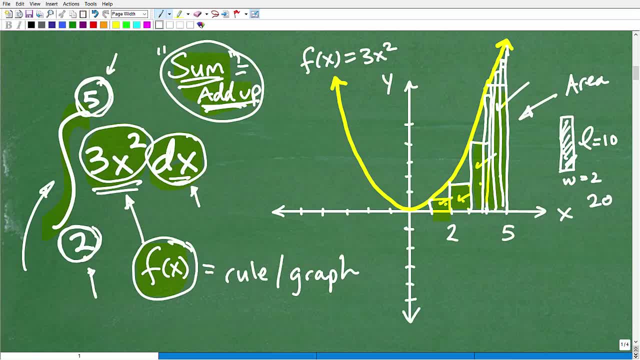 kind of make a little bit more. uh, we're actually a lot more precise, uh kind of you know, uh kind of. so now i'm still doing the same basic math, i'm still doing just length times width, but now i'm adding up, i'm finding the sum of a lot more skinnier little strips here, little rectangles. 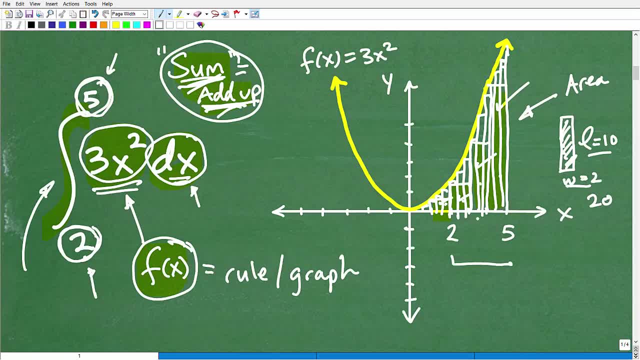 okay, that go between two and five, and i can use my little ruler and my graph paper to kind of, you know, really measure out little tiny, little skinny guys here and i measure up this way and i could, i could find a better, closer estimate of the area underneath that curve. okay, so i'm going to add up. 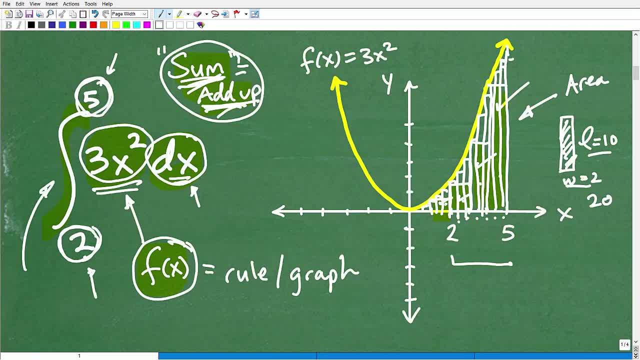 okay, that's what we're trying to do in calculus, because this shape here we don't have a formula like. the area of a square is obviously length times width. if i have a nice triangle, i can find the area. it's one half base times height, right, but this particular crazy shape right here there. 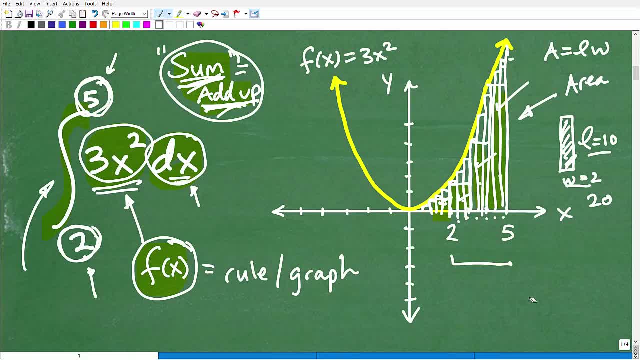 is no formula. i'm going to have to use some calculus to figure that out. so what calculus says is: hey look, in this particular problem we're going to go from two to five and we want to find the area underneath this particular curve. so we're going to add up this shape right here and 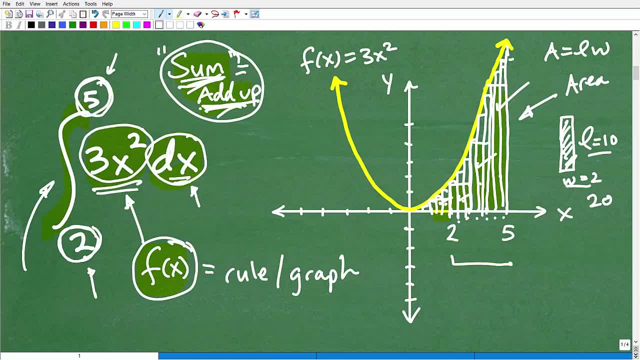 we're going to add up this particular graph, three x squared, and what this means is: add up, find the sum of all these little rectangles. now here's a deal in calculus. to find the exact answer, our little rectangles have to be infinitely skinny. i don't know if you can kind of grasp that right. 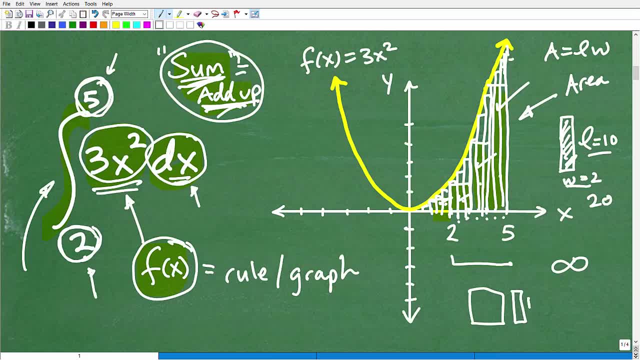 so here is one kind of rectangle. if i make it smaller and smaller and skinnier and skinnier as i make my rectangle, uh skinnier, all right, and if i can make them infinitely skinny, then i have the perfect, most like precise, exact area underneath this curve between uh two and five. all right, and that is. 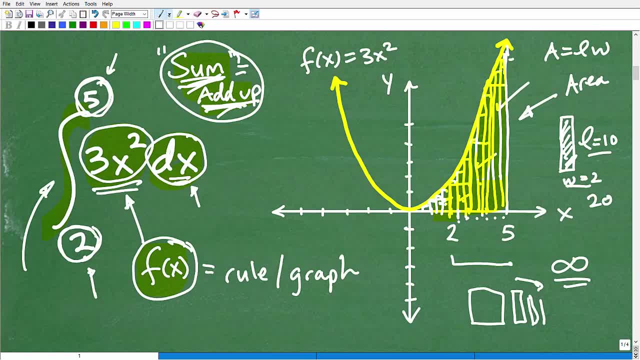 what calculus is really about. now, obviously, you know at this point, uh, the mechanics behind doing that is a little bit more involved, for sure. all right, this is where you actually need to study calculus, but it's not that difficult, believe me, it's not that difficult, but it's not that difficult. 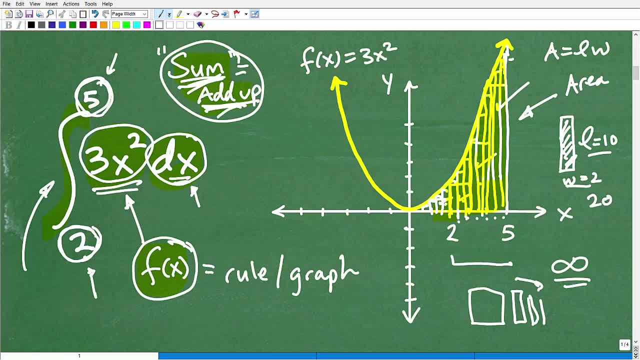 even when i tell you it's not that difficult. there's plenty of people that i would say are not like math's not their strongest subject, who were able to learn calculus and do pretty well in the subject. so you can't too, but there's a lot of you know, uh, prerequisite work they have to do. but 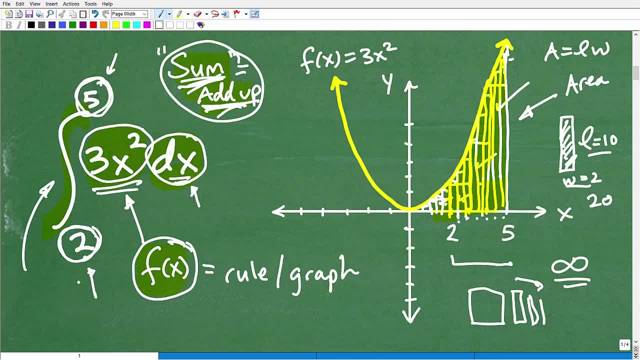 that's effectively what we're trying to do. so in this calculus notation, what we're seeing in this particular problem is a very common type of calculus problem- is add up the area underneath this curve. this functions curve between two and five, and we're going to find the sum of all these. 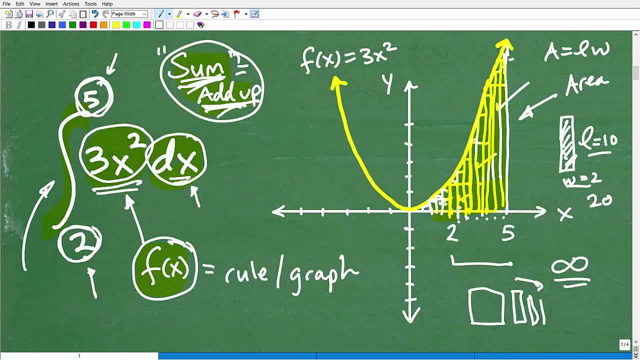 little rectangles and we're going to find the sum of all these little rectangles and we're going to find the sum of all these little rectangles and we're going to find the sum of all these little skinny rectangles. that's basically it. now, here's the good news when you study calculus- all right, let me kind of erase. 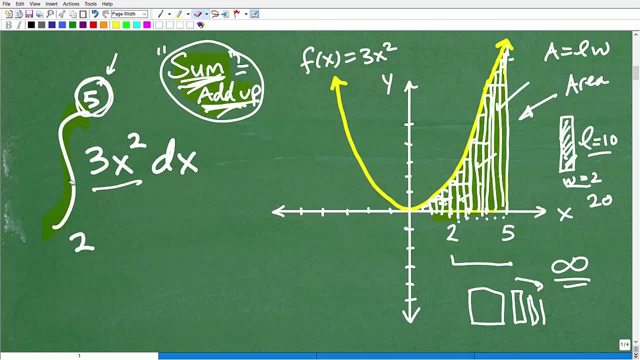 all this, you might be saying: oh, wow, you must. this thing must require a ton of different steps. uh, to do you know, like, you know, how you know, would i have to be working on this problem for you know an hour to get the answer? the um, and the answer to that question is no. okay, in calculus we have 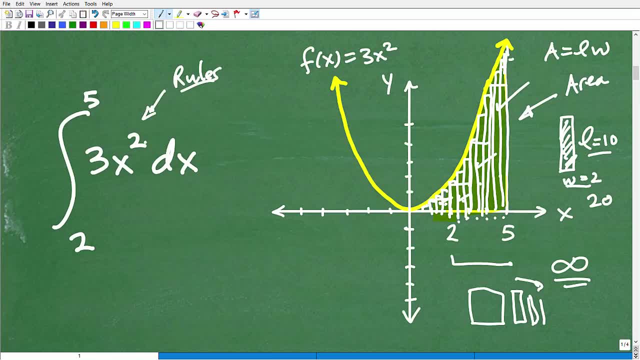 nice little rules that we can use to solve this problem, and we can use them to solve this problem in calculus. we have nice little rules that we can use to solve this problem and we can use them to solve this problem. that you learn, okay, that we can do something with this little function, and then we'll add in these. 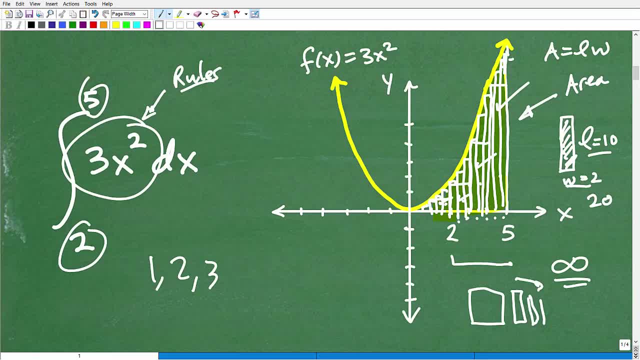 numbers and like one, two, three. it's not that bad. you will get the precise area. so a big part of learning calculus is learning these little rules and procedures, etc, etc. but what i'm talking about here is just conceptually. you know how we want to think about some of this basic notation in 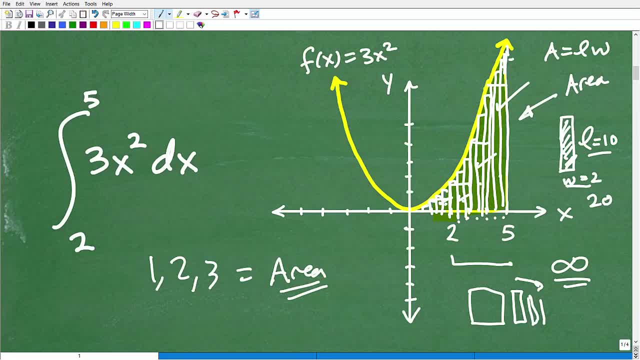 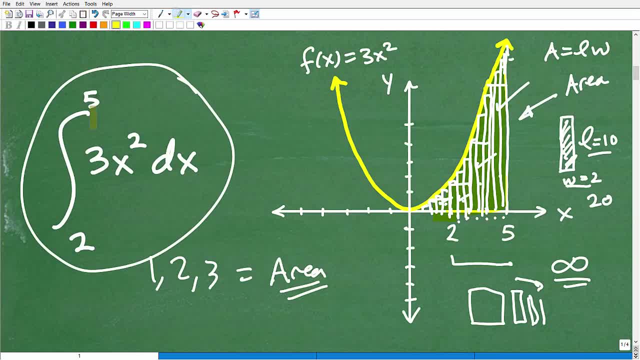 you know, and you see some crazy math. you know, look out for these symbols. you'll be like, oh yeah, that's what that means and and that's, i think the beginning of of uh, learning is is is to, you know, drop the anxiety level down by demystifying it a little bit. you know, as an introduction, 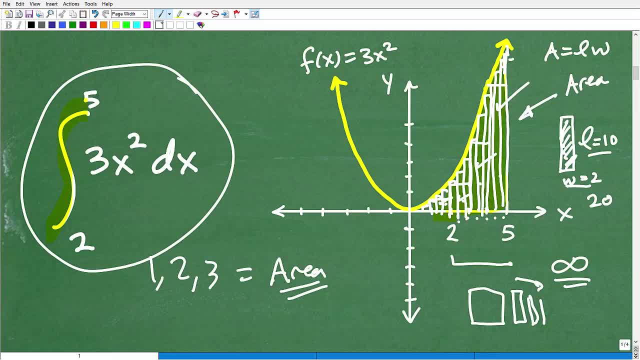 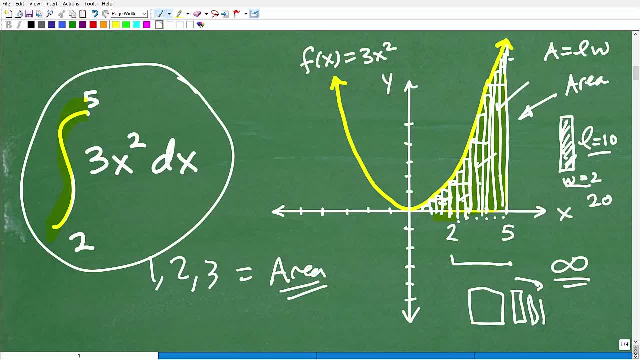 no doubt about it, and it will challenge pretty much anyone who, uh, takes it okay, but, um, you can handle it. all right, there's a lot of background work that you can build yourself up to, but you can handle it. but again, the main idea of this video is just to you know, show you that you know. 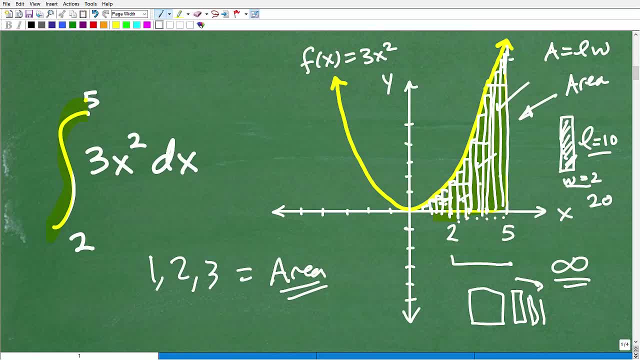 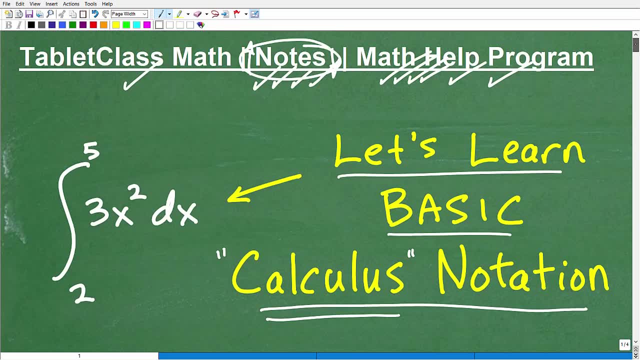 what these symbols and mathematical symbols have: meaning and practical meaning. all right, all right, so let's just call, kind of call it quits at this point and i'll see you next time. bye, bye, this point, hopefully you're like. you know, that's pretty interesting, you know? and uh, walk away from. 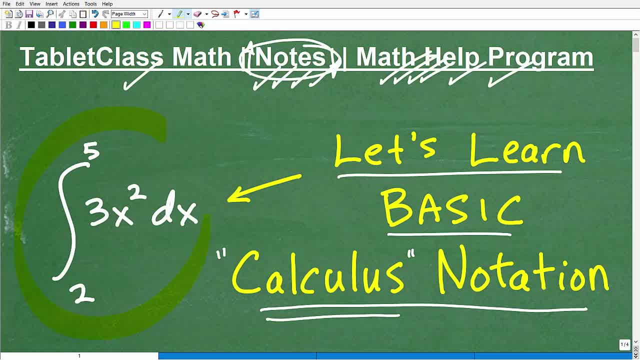 this video, knowing a lot more about calculus than i thought i ever would have imagined. so even look at this problem now and you'll say, hmm, yeah, you know what, that's not that bad. and if you do like a little google search on calculus or just look at this notation, you'll, you know, i think you'll. 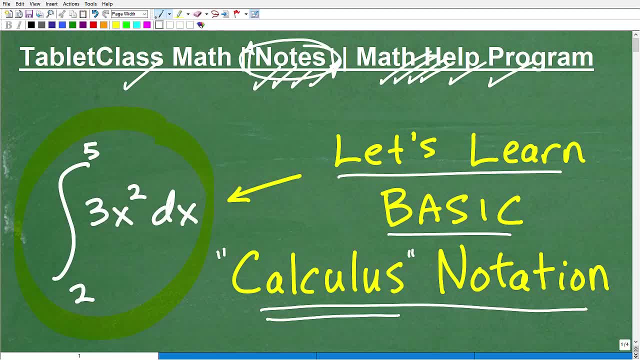 have a much better feel for what the subject is about. of course i'm you know i'm leaving out a ton of other stuff, but what we talked about here is a huge part of calculus called integration. all right, so if you found this video interesting, if you liked it in some way, please consider.